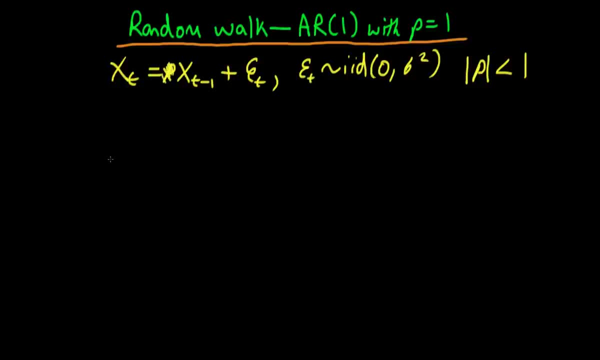 to be dealing with a non-stationary time series, but we need to think about why is our time series going to be non-stationary? And in order to do that, the best thing to do is first of all to back substitute in for xt. So if we back substitute in for xt, we get that xt is equal to xt minus 2. 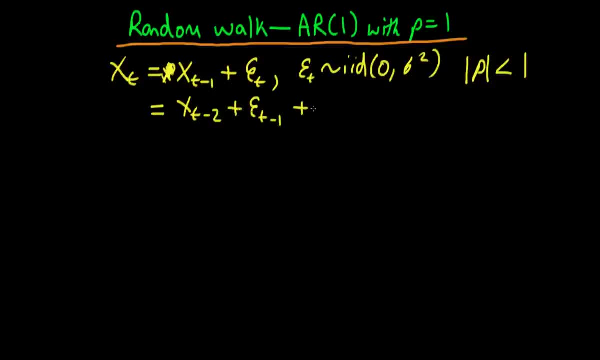 plus et minus 1 plus et, And then, if we were to continue doing this all the way to the first period, we would get that xt was equal to x0 plus the sum from i equals 0 to t minus 1 of et minus i. 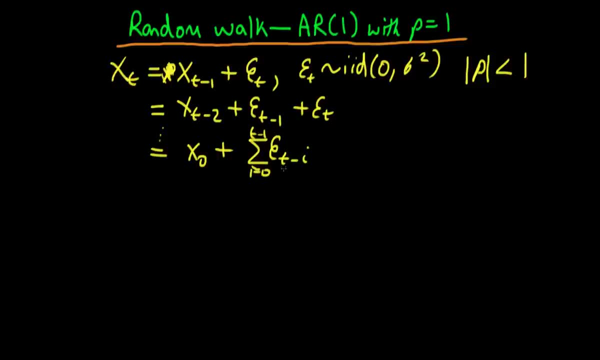 And we could get the second term just by doing this, Noting the fact that we add on an extra et term for every sort of extra back substituted value of x which we go back to. So we've got that xt is equal to x0 plus this sum term here. So now we're. 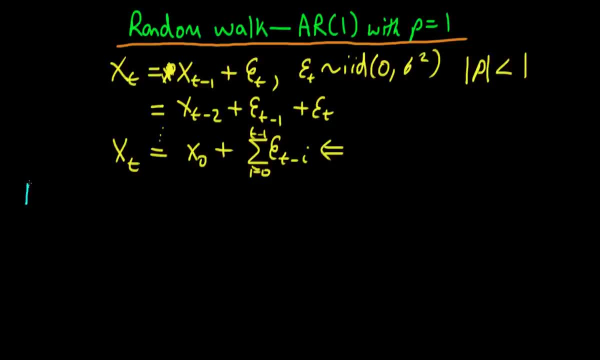 in a position whereby we can think about the properties of an AR1 process with rho equal to 1, which we call a random walk. So the first property is that if we look at the expectation of xt, we can see that it's equal to the expectation of x0 plus the expectation of this second term here. 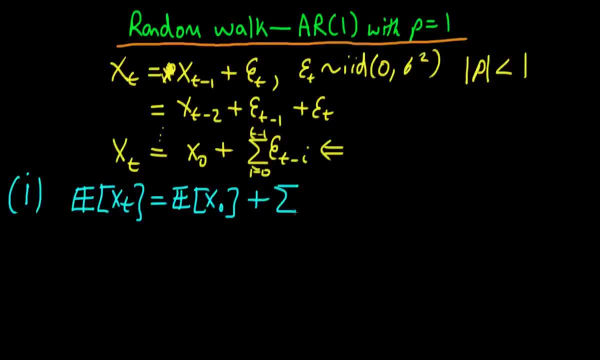 But this second term here, if we just write it out, it's going to be the sum from i equals 0 to t minus 1 of the expectation of et minus i. And since we know that each of these ets is iid with a mean of 0, this second term goes: it's all equal to 0.. So we've got the expectation. 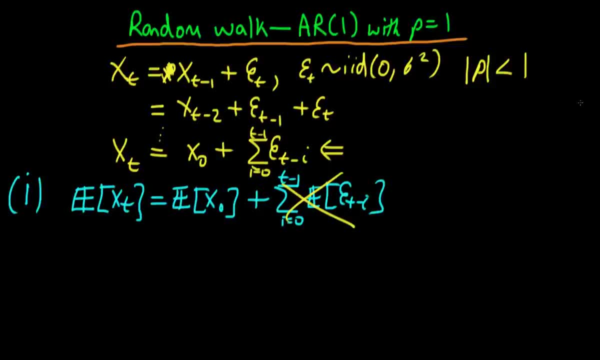 of xt is equal to the expectation of x0.. Well, that's easily dealt with, just in a similar way that we dealt with it previously. We just set the expectation of x0 equal to 0. And then that implies that we have the expectation of xt, which is equal to 0. So we have a process which is: 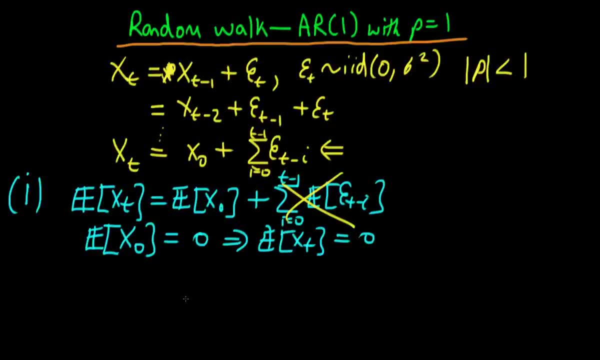 constant in mean. So it's not the case that a random walk is not constant in mean. It is actually a constant in mean process. So it's not non-stationary, It's not a constant in mean process, It's non-stationary. for that reason, Then if we look at the second condition, So we need to look. 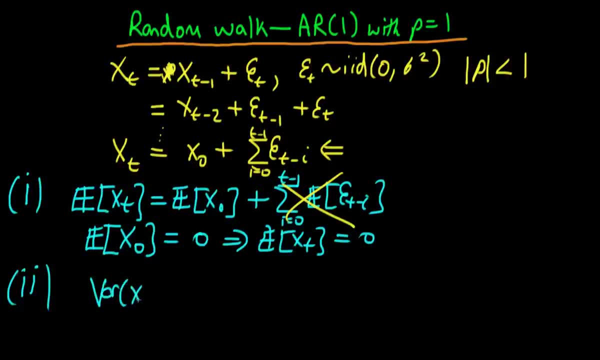 at the variance of xt now. So if we look at the variance of xt using this particular relationship which we derived down here, Well, that would be equal to the variance of x0. But if we choose x0 as just being given, it's just a constant- We can sort of think about it as not having a variant. 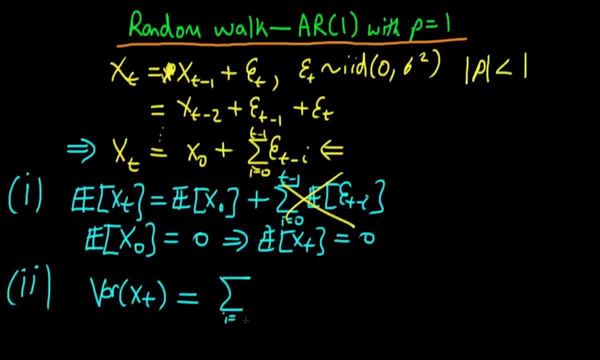 So then we have that the variance of xt is equal to the sum from i equals 0 to t minus 1 of the variance of epsilon, t minus i, And notice that we don't have any covariance terms when I take the variance operator from the outside to the inside, because of the fact that our et are independent of one. 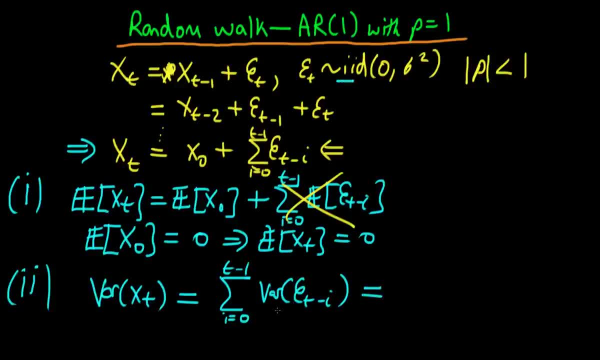 another. So then we notice that the variance of each of these terms is just sigma squared, And we've got t of them, because this sum is starting at i equals 0 and going all the way up to t minus 1.. So we've got that the variance of xt is equal to t times sigma squared. 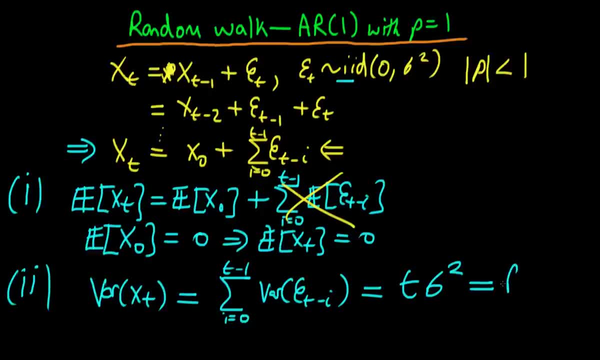 And notice that this isn't a constant. It's a function of time. Hence our process is non-stationary because of the fact that its variance isn't constant. So that's the reason that a random walk is itself a non-stationary time series. And let's look at the third and final condition. 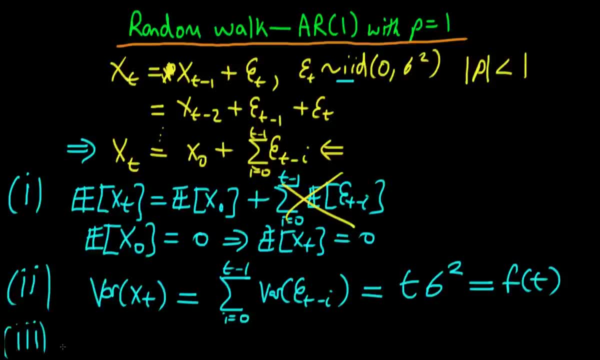 for a series to be stationary. So here we're looking at the covariance between xt and xt plus h, And in order to do this, we first of all note that we can just write down straight away what the relationship between xt plus h is with xt. Well, xt plus h is just equal to xt plus the sum. 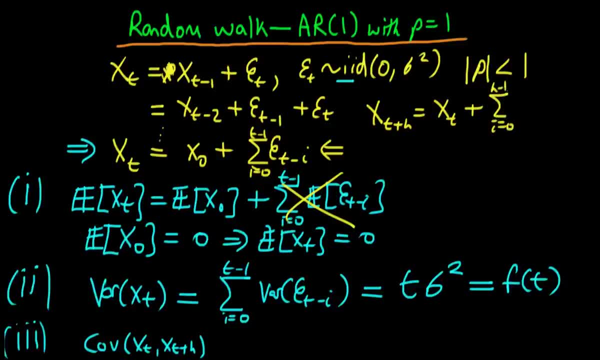 from i equals 0 to h minus 1 of et plus h minus i. So if we just replace xt plus h with this particular term here, we have that the covariance of xt with xt plus h is equal to the covariance of xt with xt plus this sum. here where the sum goes, 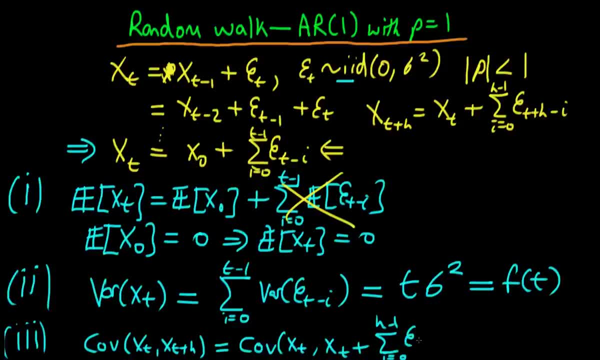 from i equals 0 to h minus 1 of et plus h minus i. And finally, we note that there is no covariance between xt and this error term here because of the fact that these errors are independent, So we can just get rid of this term here.